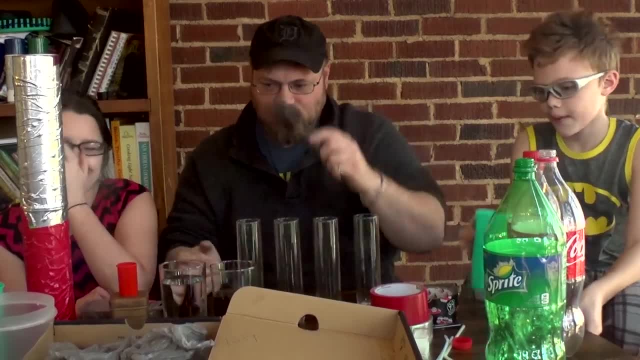 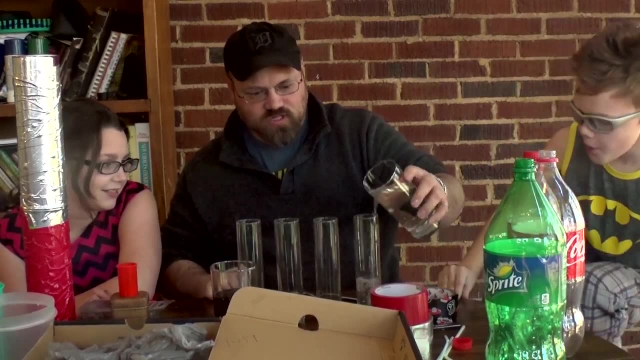 We're doing it for a video, Yes, and these, you can put water in them to different levels. So the first one, you kind of want to fill it up just a tiny little bit. The next one, you fill it up a little bit more. 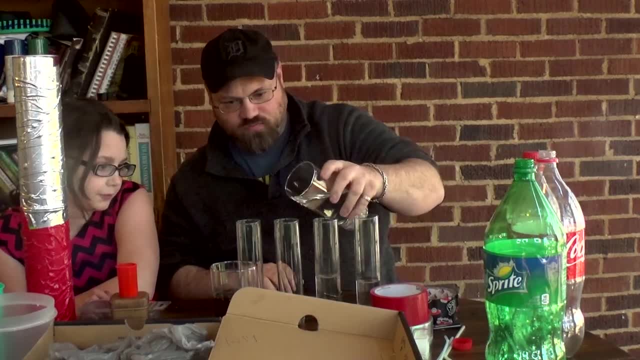 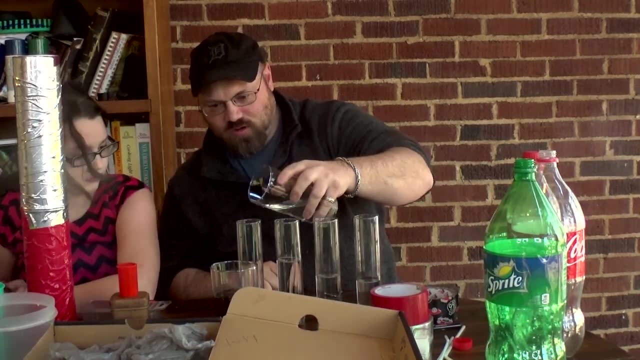 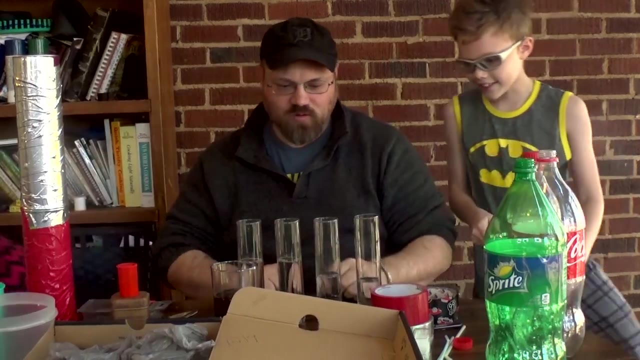 And the next one: you fill it up a little bit more than that. And the next one: I'm probably going to need more water. You fill it up. Oh, I am going to need more water. Can you go get me some more water? 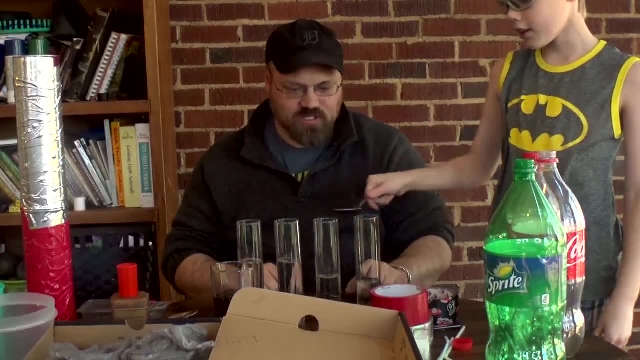 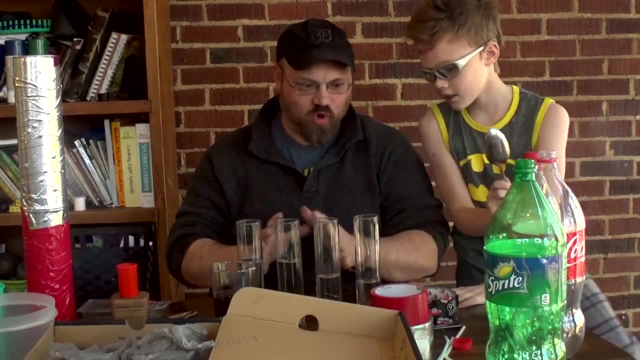 Yeah, you're going to need to fill it up some more. So what happens is this one should make a higher pitch note than this one. But wait, you're spoiling it because we don't have it filled up. Okay. 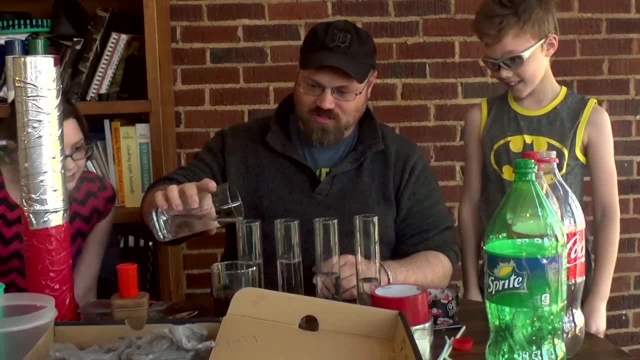 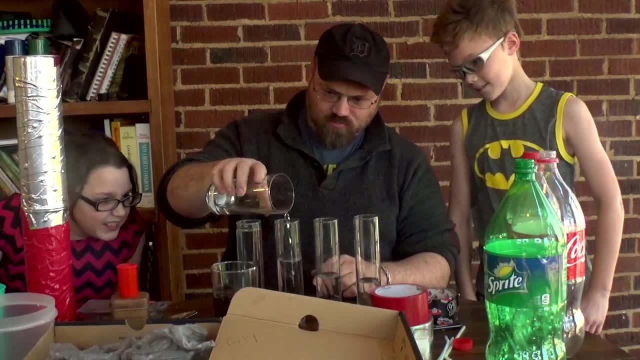 Okay, We haven't filled it up yet. Now I don't know if it will actually work with these glasses or not, but we will. So there you go. Let's put a little bit more in this one. I'll put it in the rest. 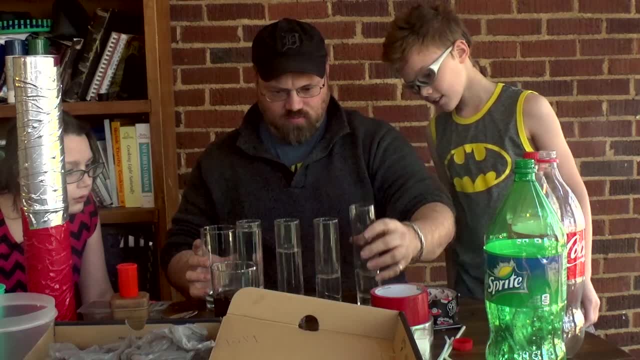 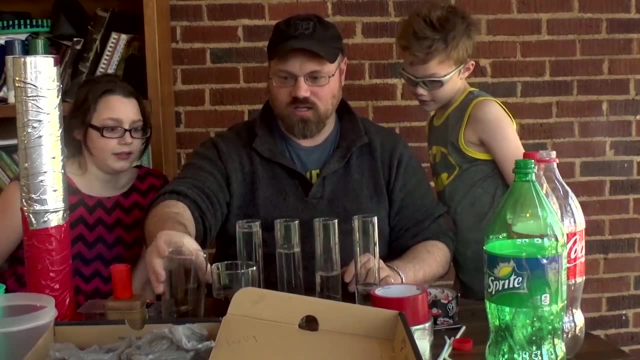 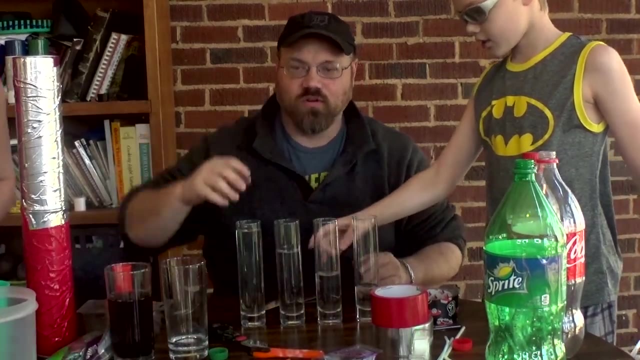 And let's see There. You want it to be clearly different with each glass. Yeah, kind of like stairs. Yeah, I think our cardboard box might be kind of in the way. That's for another project. Okay, You want to ding it? 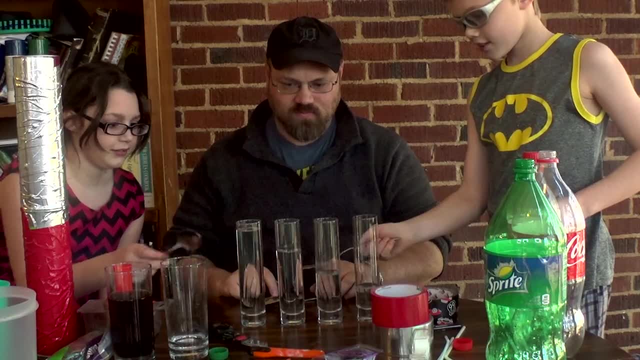 Sure, They are different, sounds huh. So then, when you have enough, Now you can do it with more than just these. Like Etta, go fill this one up again. Dad, you hit that one and that one, Okay. 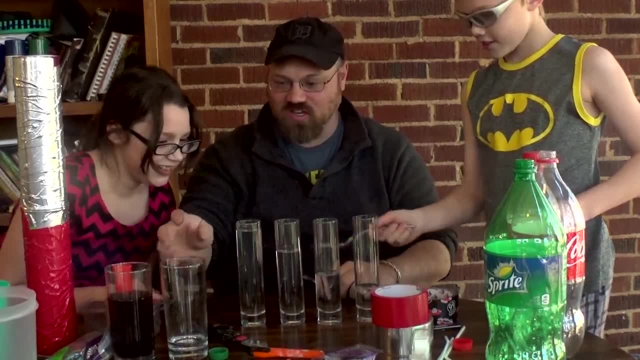 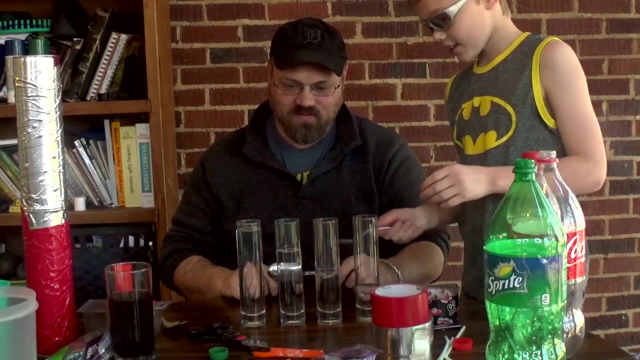 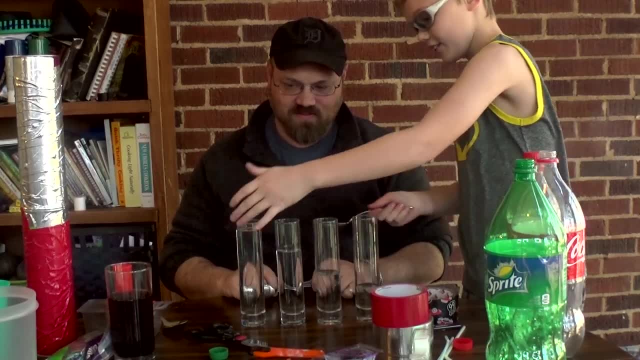 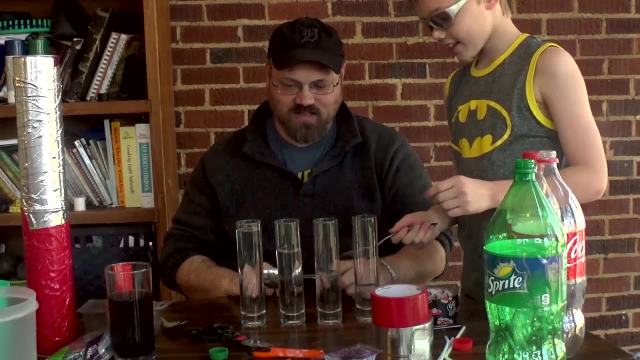 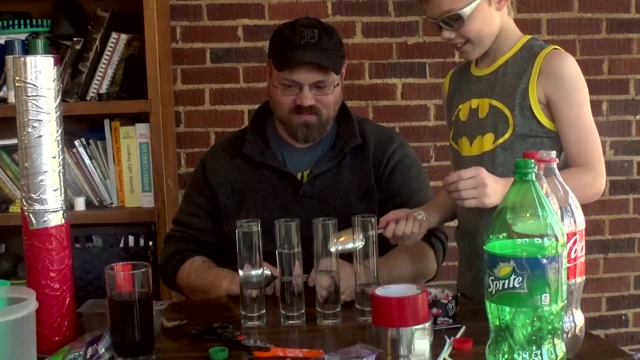 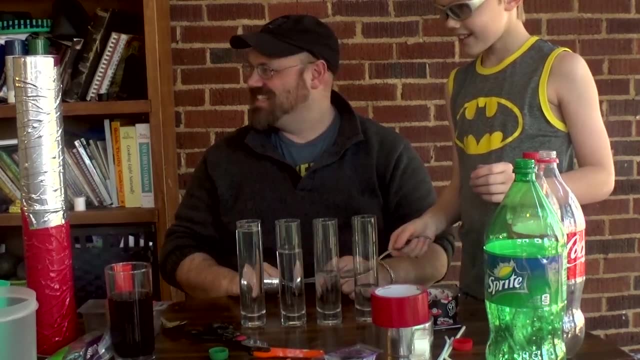 That sounds cool, That's neat. huh, Bring the other one over. Wait, listen Now this one. I think will be really deep. Listen, Listen. Can I try that one? Yeah, Okay, Let me try. Whoa.